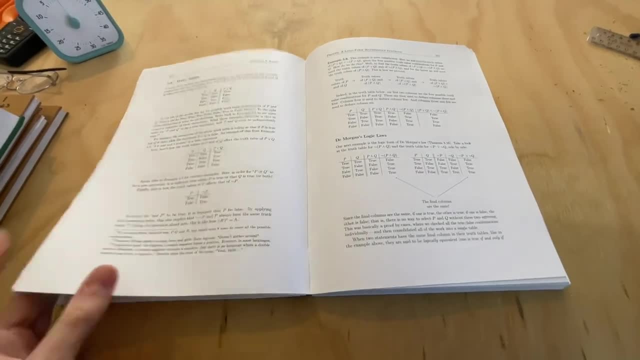 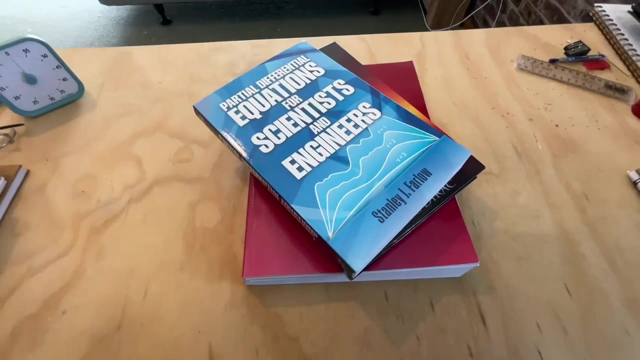 But I will give you an example. So this is a really awesome thing, because lots of cheaper books typically do not have that latex typeset. I'll give you a couple of examples of cheaper books that are not printed in latex. So this one right here is a very popular book on Amazon. 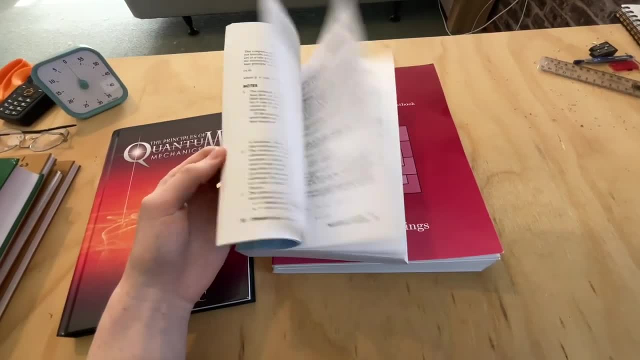 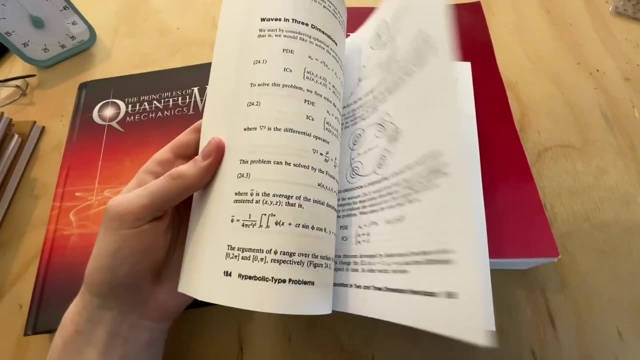 It's on PDEs and this book's okay. I mean, it's not too bad, I'm not. I think it's okay, But, as you can see, it's definitely not printed in latex. As you can see, the equation is not printed in latex. 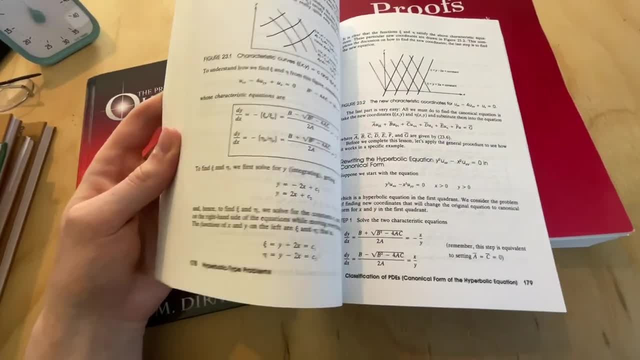 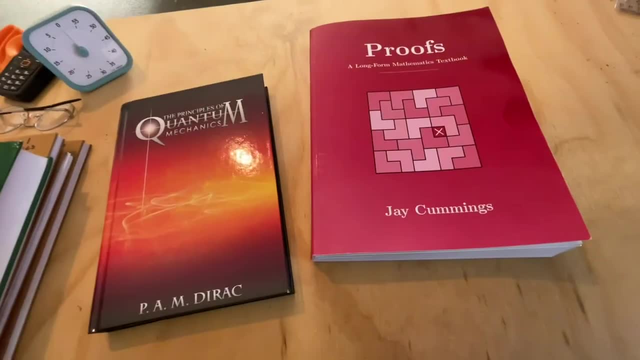 The equation formatting is doesn't look very good. I mean, it's not as bad as some of the others, but it's still not. it's still not that great, but it is a cheap book. And secondly, we have Polderak's Principles of Quantum Mechanics, So this is a very cheap. 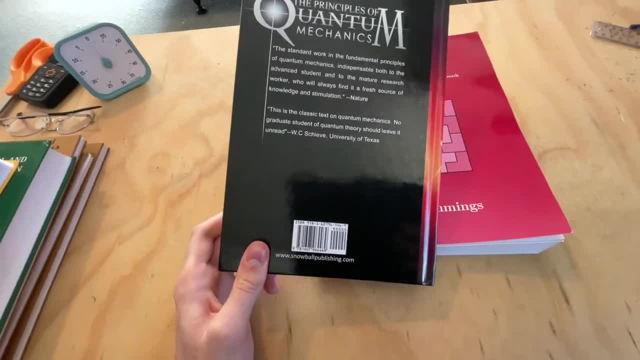 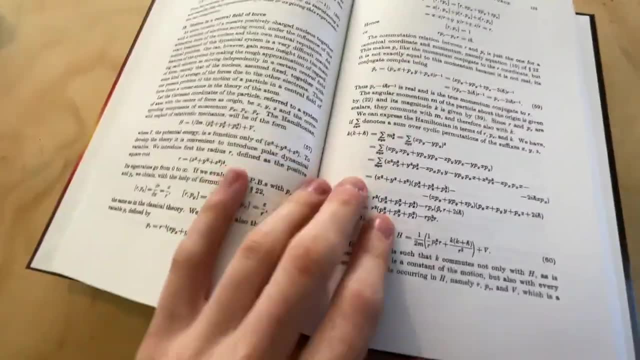 hardcover. I picked this up for like only about like $50, New Zealand dollars, so it is a really cheap book. As we can see, the printing, the equation formatting on here is awful. It's really really small. It's hard to read. 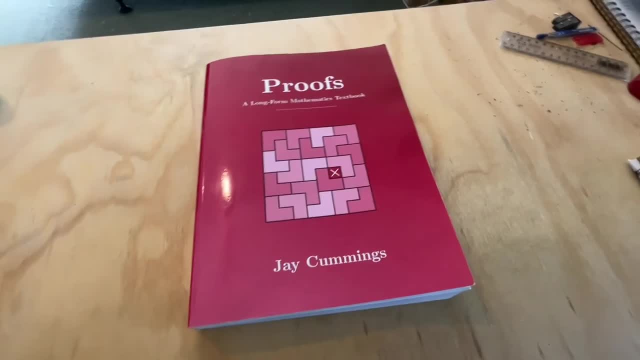 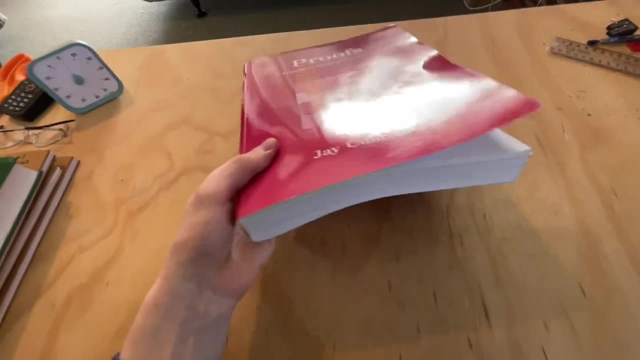 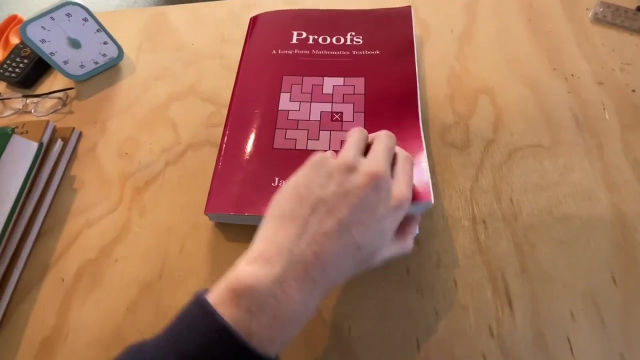 So the fact that this is printed in latex is actually a really good achievement- the fact that he managed to do that. but physically speaking this book is quite hefty. It's a big book. I don't exactly know how much it weighs, but it definitely is a big book. I mean, the pages are quite thick. This book in 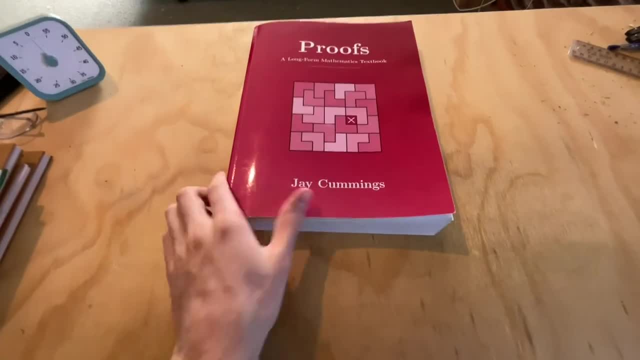 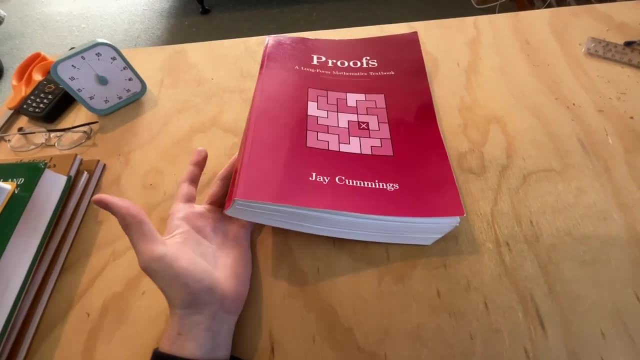 total is about 500 pages, So I mean fairly standard, but it's it's definitely a big book. It's very hefty and so much so that they're binding of this book really, really strongly. I've read reading about Polderak since we were here less than 90 years ago and I'm really motivated to make a final copy and então thirsto. 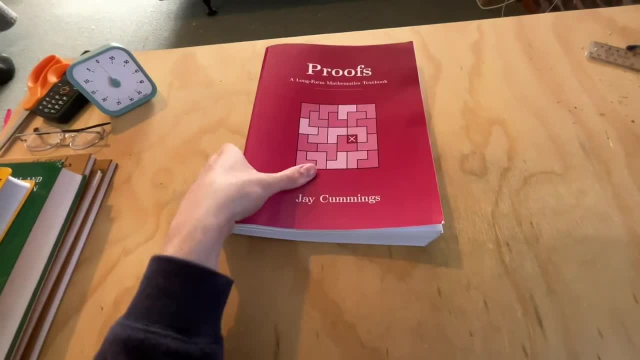 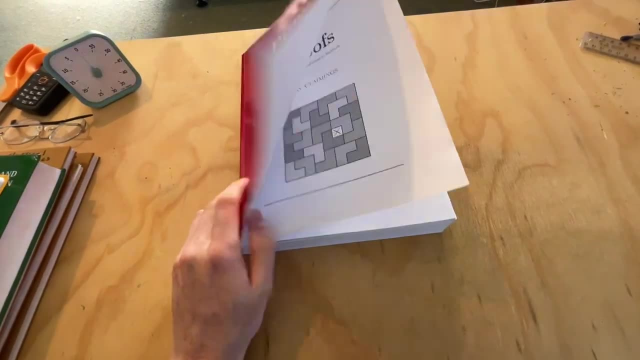 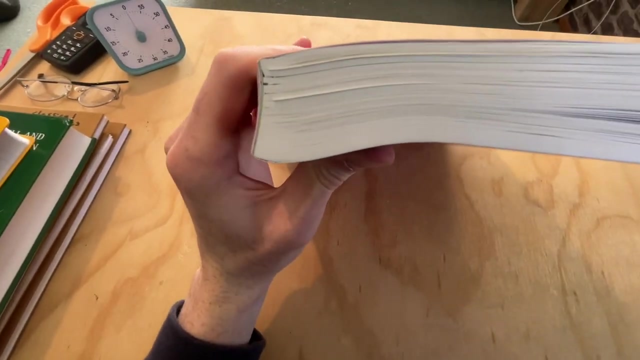 and that's where I have the complaint- is the fact that to hold a book of this weight using such cheap binding just doesn't work. I just, I mean, the book is still physically bound together, as you can see, but it's really struggling. I mean, look at this binding. it's just this tiny little bit of glue. 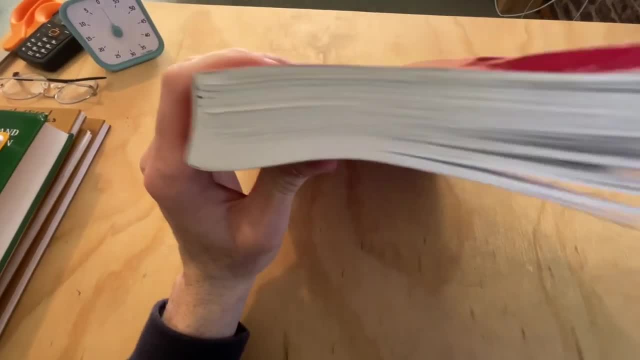 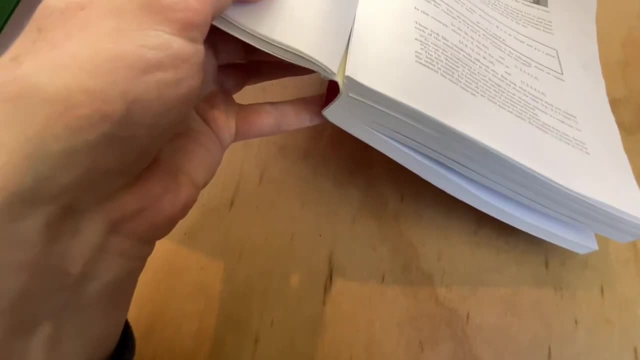 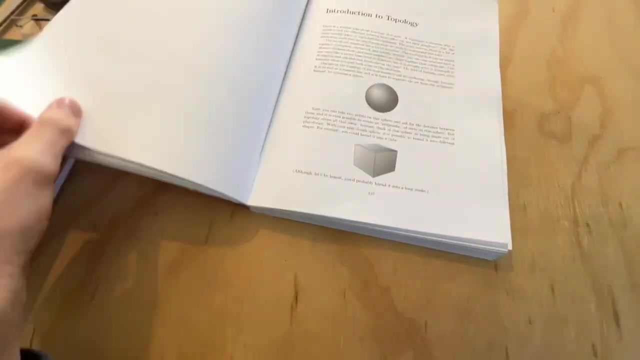 and, as you can even see, a lot of the pages or some of the pages are even falling out, like if I open the book, see, literally look, the pages are just coming away at the binding, which is really annoying if you actually want to reread this book or go through it again it. 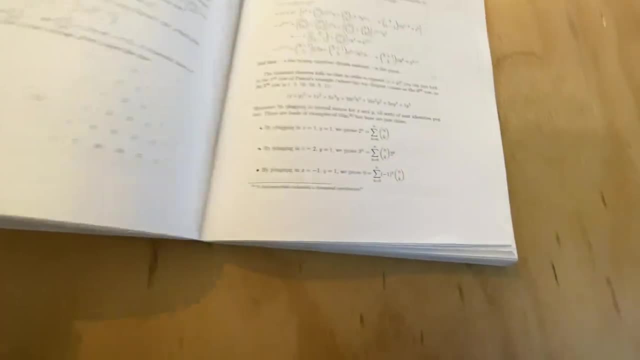 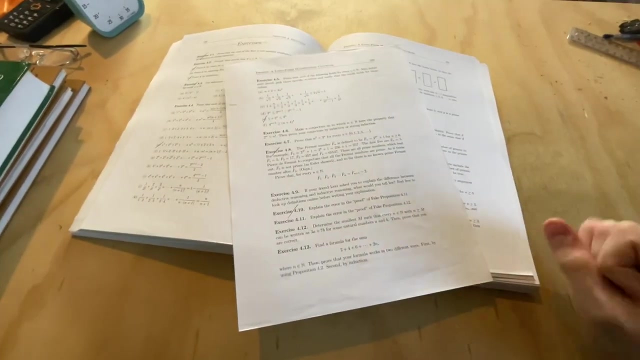 makes it very difficult. as you can see, at some places the pages have even literally just come out. so, yeah, very annoying and yeah, I would. I understand that he wants to keep the book cheap, but I mean, surely he could improve this binding. I don't know if he's going to be able to keep the book cheap. 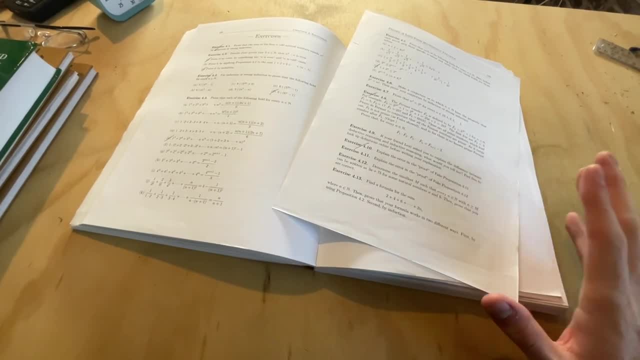 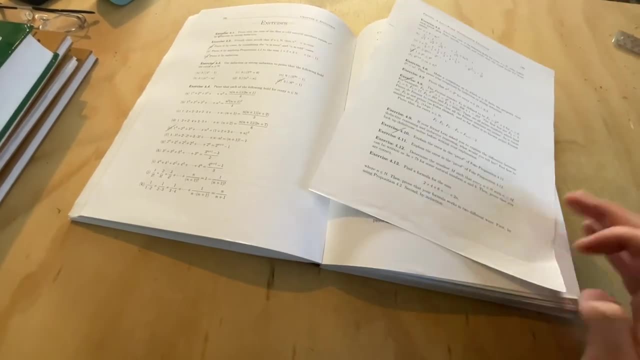 I don't know if he's going to be able to keep the book cheap- I mean it's just- or offer a hardcover option, because having a book of this size and such cheap binding just to me just doesn't seem like a good idea. it just, it just doesn't hold together. 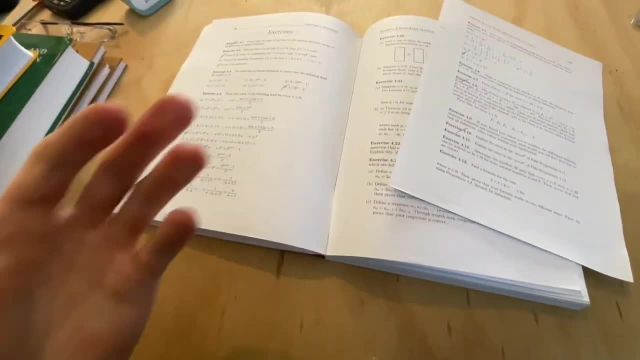 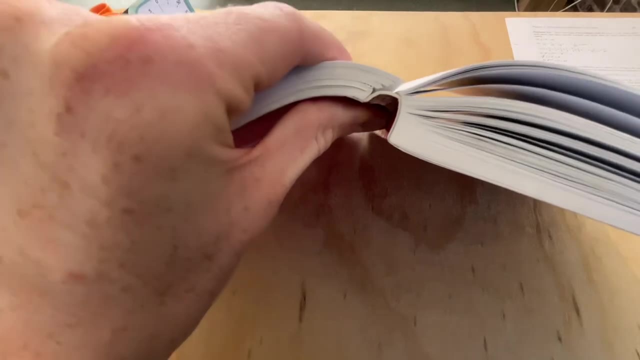 as you can see, especially if you're the type of person to sit with your book and say: have your arm on it like this- not a good idea. if you do that, you'll end up with with this. as you can see, the the pages are literally just coming away from the binding. so, other than that, let's get into the book. 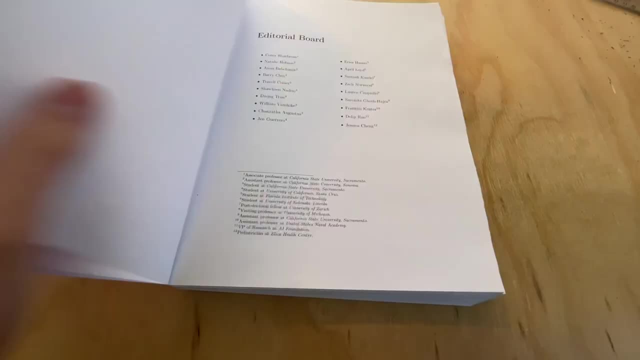 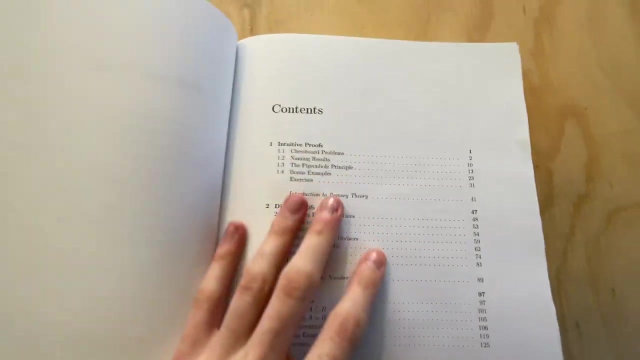 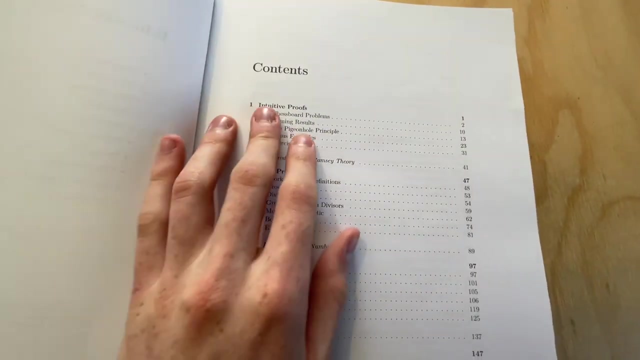 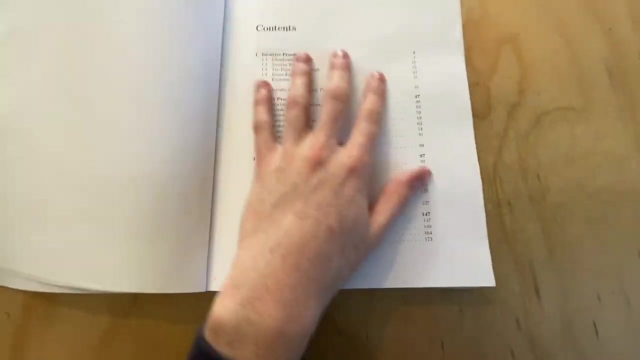 it's tabler content. so first up, we've got intuitive proofs. now I absolutely love the way Cummings has- uh, late has- set out this book. it's incredible. there's so many cool things he does um so intuitive proofs. talks about the pigeonhole principle, but yeah, just really, this book is very. 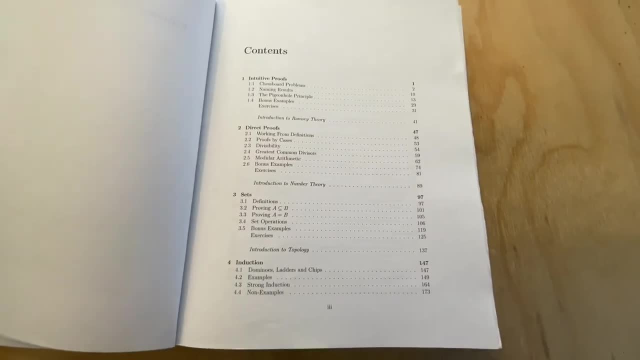 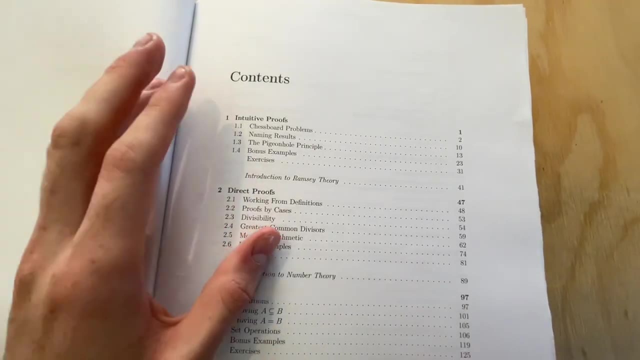 pedagogical. he has an incredible style that is totally beautiful and he's got a lot of different from most, um, traditional mathematical textbooks. a lot of his stuff is very conversational. it's really easy to follow, honestly, if you've just got a little bit of calculus and just a math. 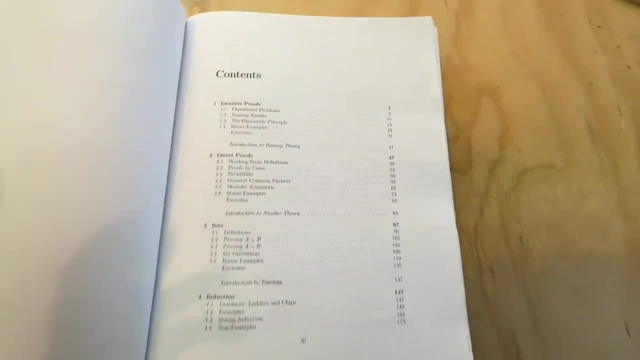 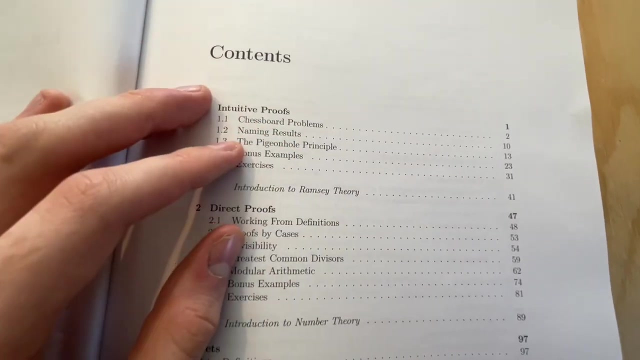 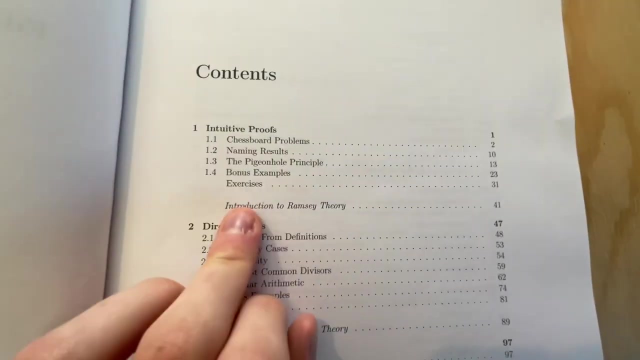 background, you can pick this book up and learn how to write proofs. so, yeah, really cool. he has this chessboard problem and then he talks about the pigeonhole principle- really awesome. chapter um, and in between each chapter he has an introduction to like some field of mathematics. so here we've got Ramsey theory, number theory, topology. 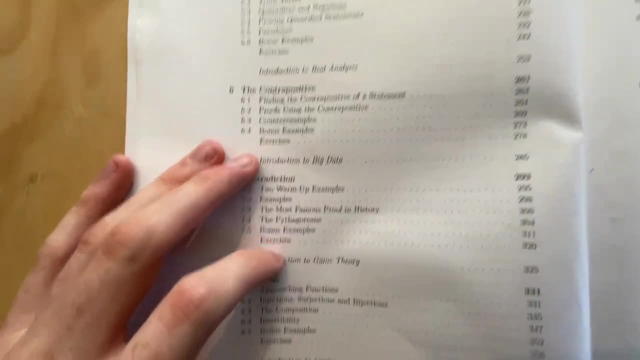 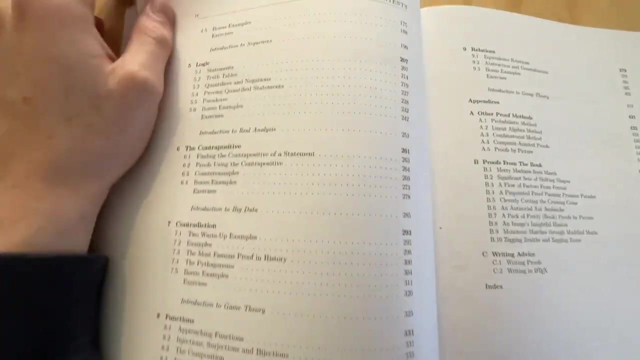 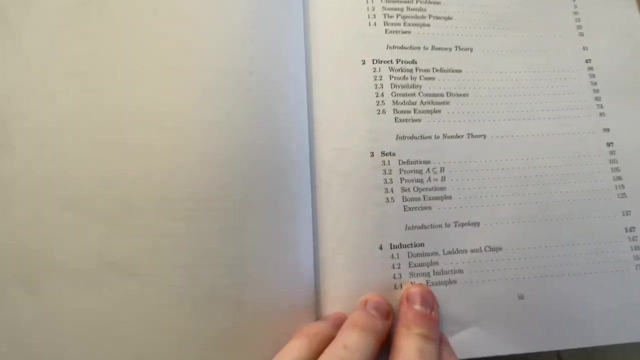 sequences, real analysis, big data, game theory, cardinality and group theory. so all these awesome areas of mathematics are most notably probably real analysis, game theory, group theory and number theory and topology. so it's really interesting that he's added these quick introductions. 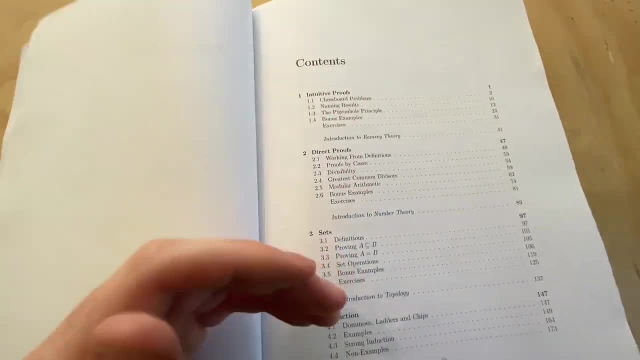 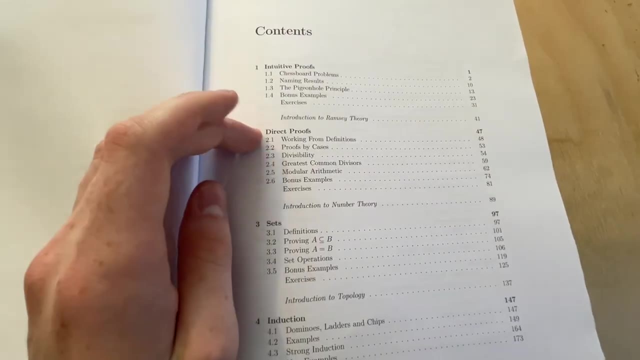 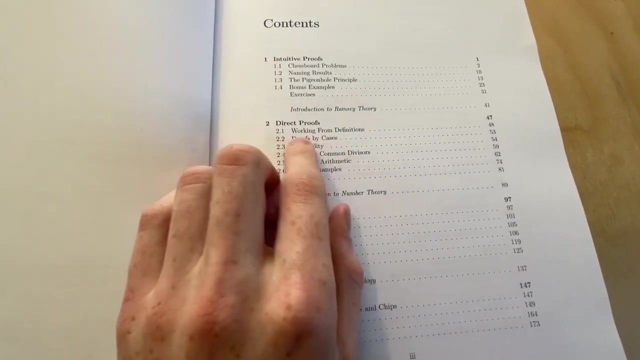 and they are generally a very natural continuation of the chapter um, so they're just really awesome. I think it's incredible he's added that in this book, chapter two, we've got direct proofs. so this is more about modular arithmetic and divisibility and, of course, he talks about proof by cases, which is a very fundamental method of proof. 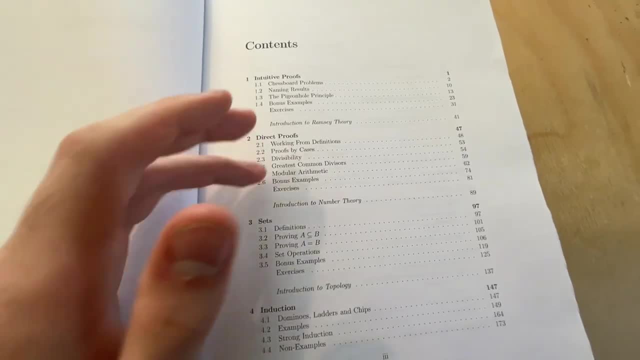 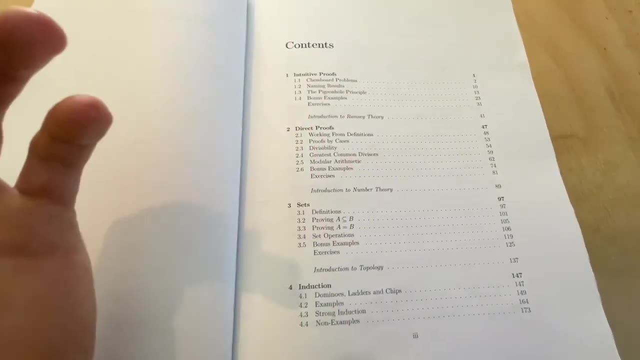 this is a really cool chapter because it's quite simple, uh, when it talks about um, just even and odd numbers and divisibility and just directly proving different things like, um, the square of an odd number is odd and all that kind of stuff. so really good chapter i. 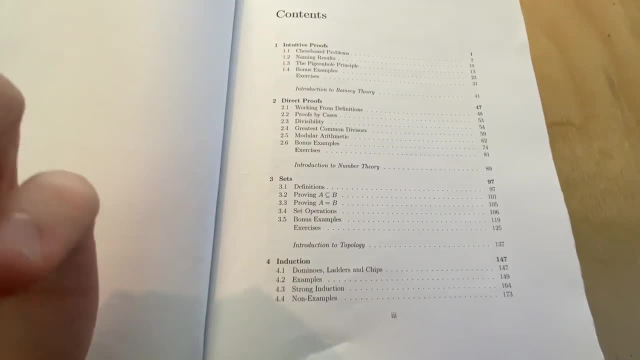 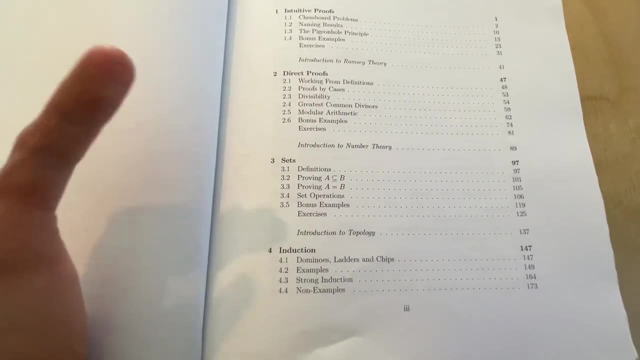 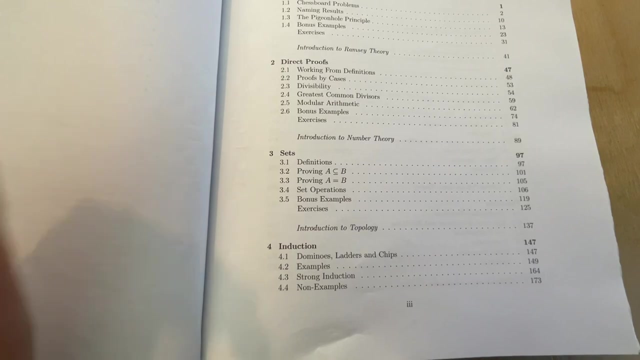 mean the module, the modular arithmetic is a little bit more tricky, um, but yeah, fun. it's a really good chapter. i really enjoyed it. uh, sets, so we move into set theory more specifically. it's naive set theory and this is a really good introduction to sets. i mean it's not conclusive, uh, specifically. 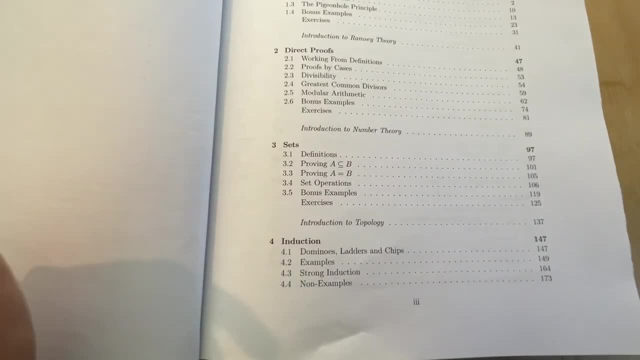 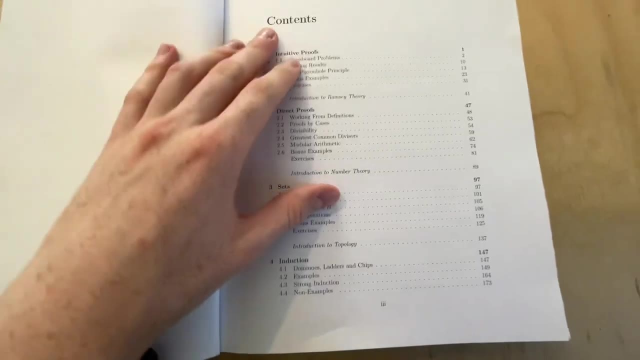 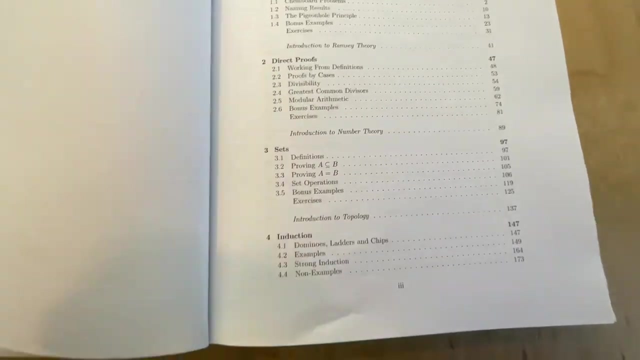 if you want to learn more about sets and set theory, i'd rather recommend a book like um uh paul harmos's naive set theory. but at the end of the day, books like this, especially on proofs, should really motivate you, give you enough information that it motivates you to go out. 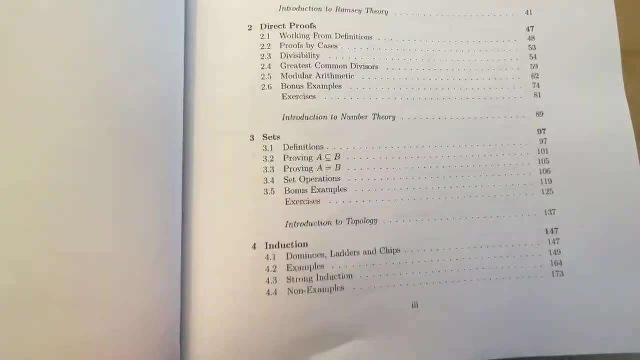 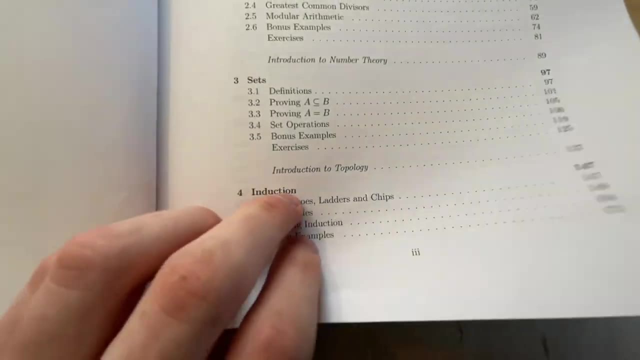 and read more. so good introduction to sets really just gives you all the basics and some really fun proofs. i really did enjoy this section on sets. i've got introduction to topology, so next we're got induction. so another fundamental method of proof. induction is quite a fun method of proof. 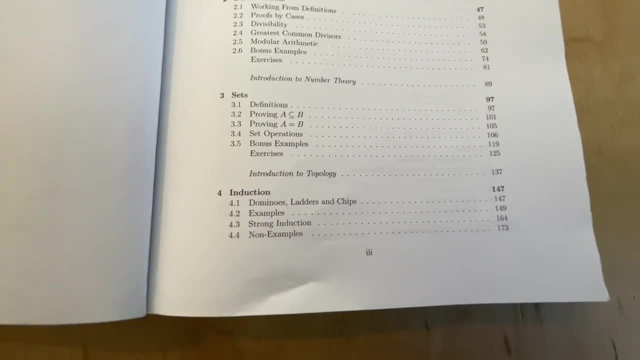 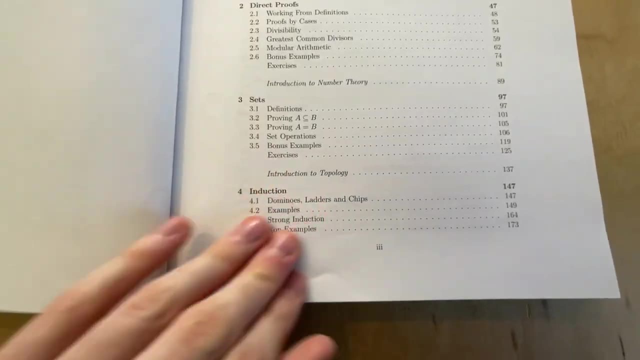 and he gives some excellent analogies. as i said, once again, extremely conversational style. um it more feels like you're literally just conversing with someone, like a friend. it's, it's really fun. um, the examples he gives are strong induction, of course, and the difference between 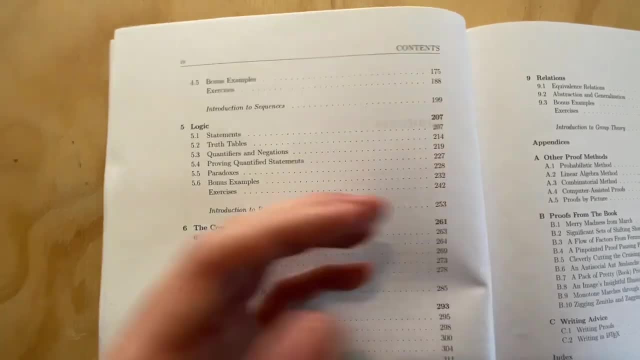 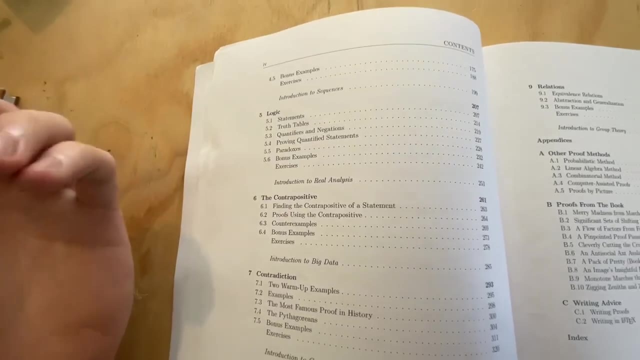 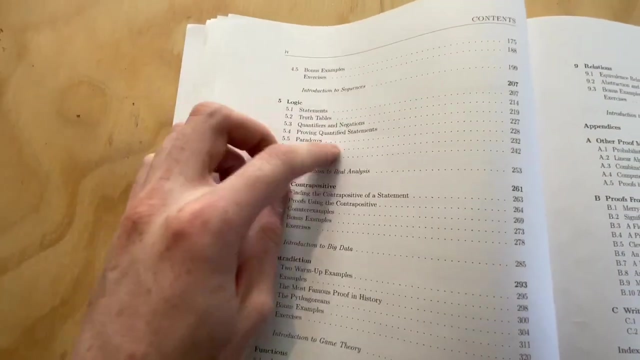 them um logic. so another introduction to logic. once again, this is a huge motivator for you to go out and learn some more formal mathematical logic. um, even more so, if you're interested, some more like applications to philosophy, like philosophical logic. really fun chapter. thoroughly enjoyed it. lots of humor in this book too, especially in the 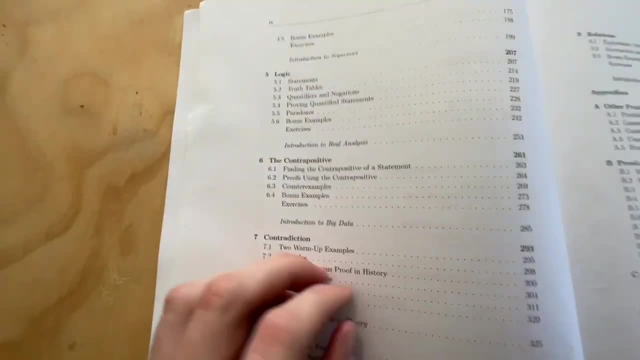 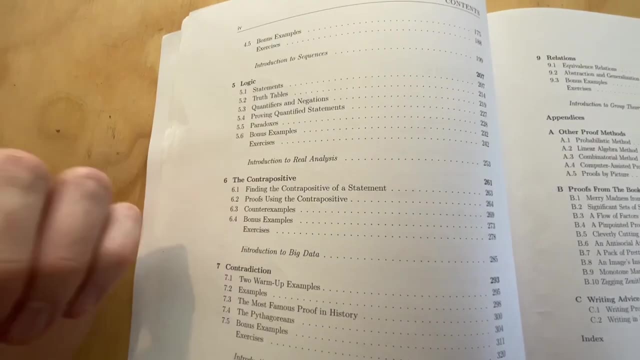 footnotes really like great humor. he's got a great sense of humor, this guy. lots of memes too. i'll show you in a moment number six, the contrapositive. this follows very naturally from logic, of course it's a concept within logic, um he uses the contrapositive to prove um various different. 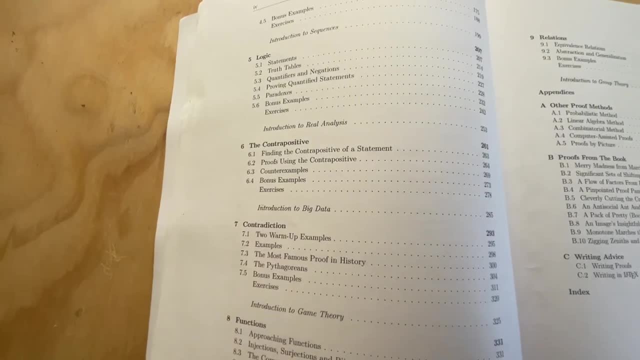 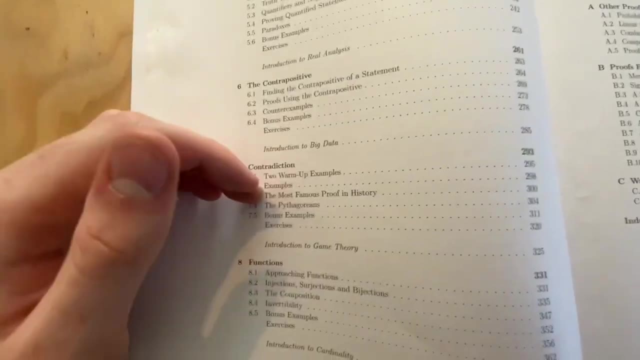 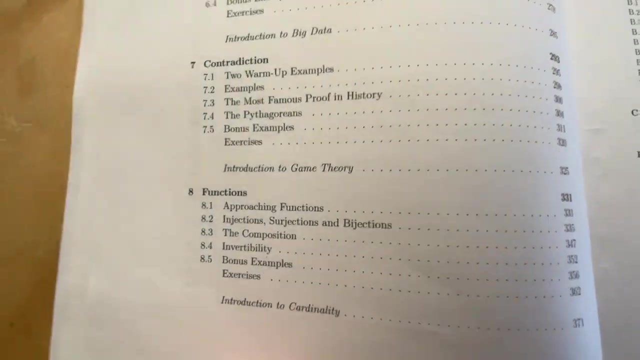 things really awesome, really great proof method and he illustrates it extremely well. next up contradiction: it's not a really fundamental method of proof. he talks about some really cool stuff in here, like euclid's proof of the infinite prime numbers and the pythagorean theorem functions, so this is more of an abstract. 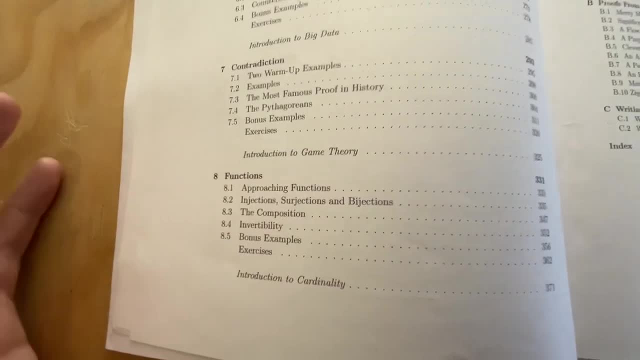 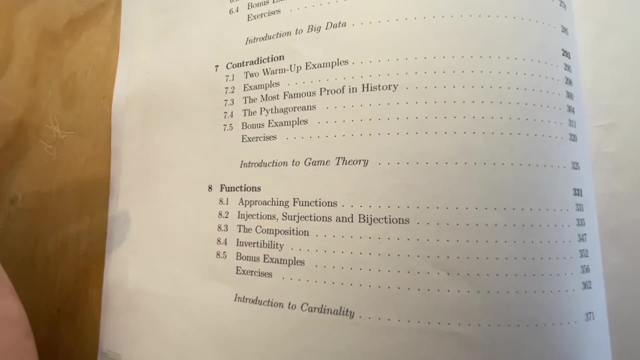 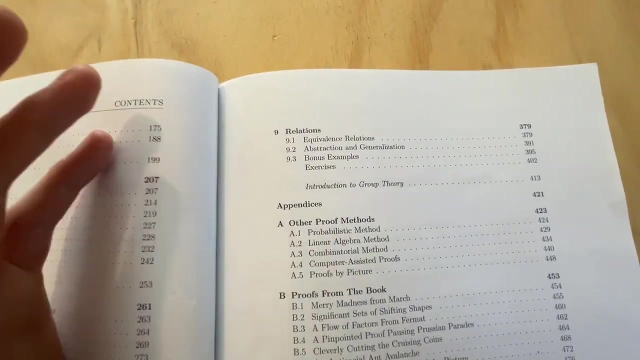 sort of chapter concepts in here, really cool. he illustrates them extremely well, really always just easy to follow. anything in this book, um talks about injections, surjections and bijections and invertibility. lastly, we've got relations, so this is where he kind of completes um the uh, your understanding of functions, that kind of stuff. 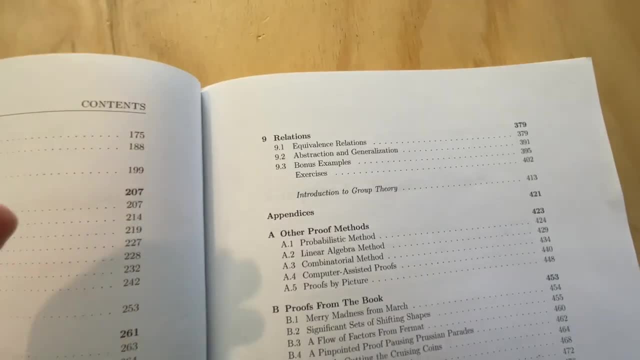 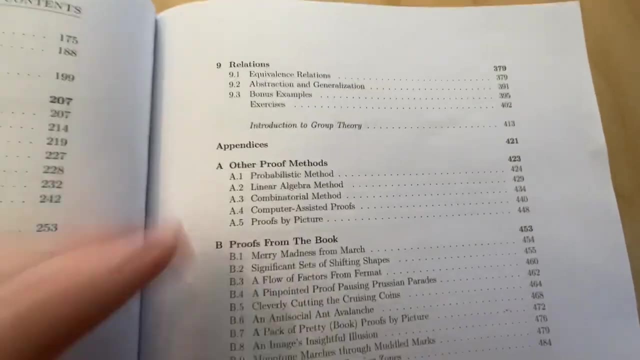 and just it's more of an abstract sort of chapter, but still, regardless, it's a really awesome chapter. i absolutely loved it. and then he has some appendices. first of all, we've got other proof methods now. this is actually a really good thing to read, especially when it comes to the linear 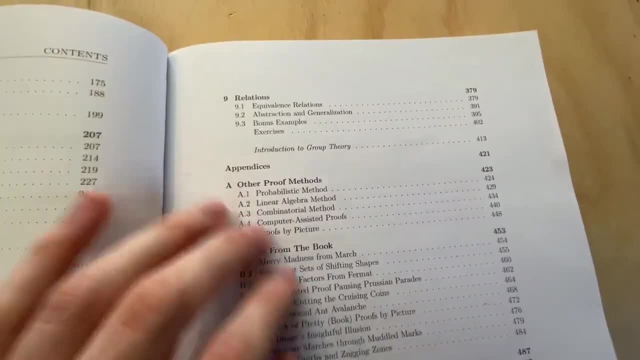 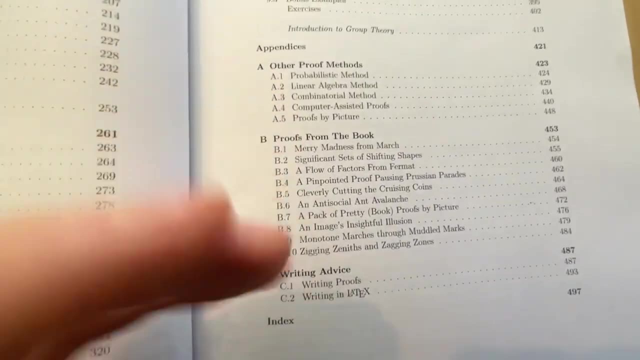 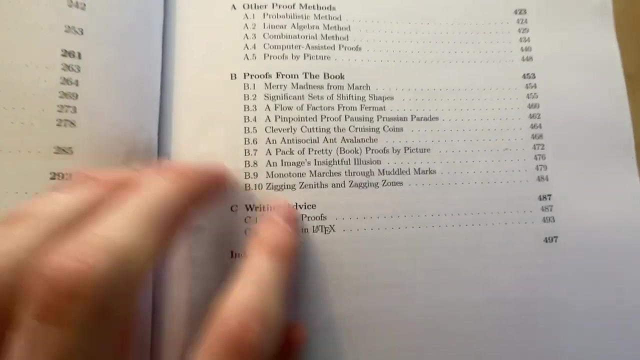 algebra method it's. it's a really good um appendix. to make sure you read these appendices um proofs in the book. these are really awesome. i absolutely love these. and, of course, at the end he's actually got some writing advice for latex, which is really cool, and i actually did learn some from this when i'm writing up my latex documents. 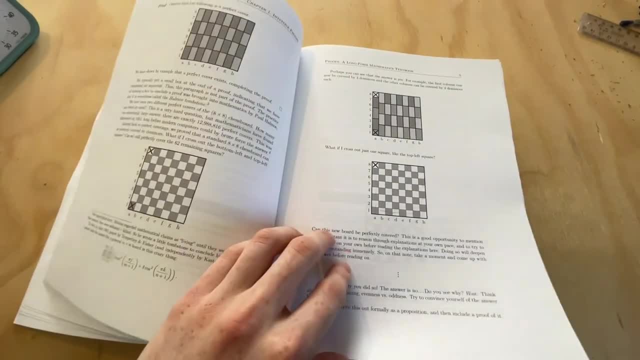 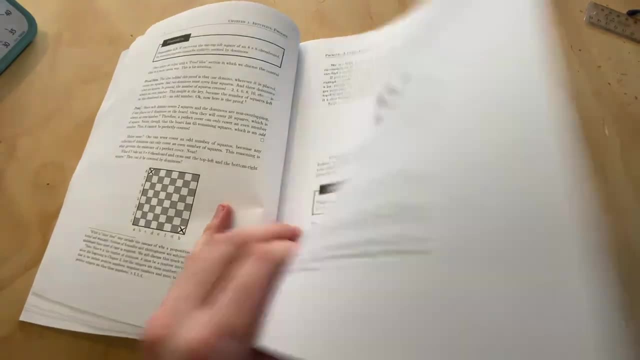 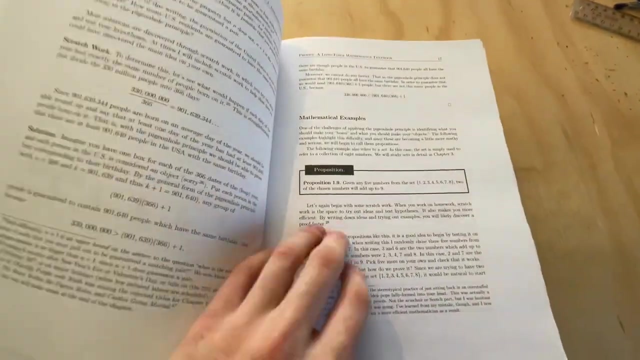 so, once again, extremely intuitive book, really interesting. um, you trust me when i say you will thoroughly enjoy this book. if you, if you even have the slightest interest in mathematical proofs, i'd highly recommend you pick this book up. with regards to the exercises in this book, so each chapter of 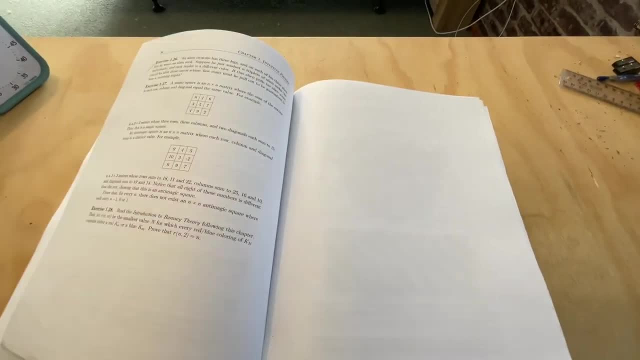 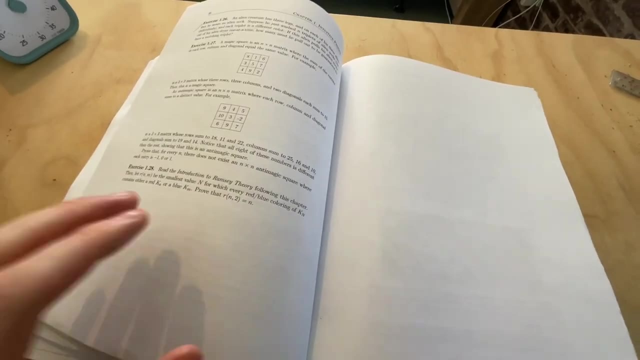 got 28 exercises. some of them have up to 50 exercises, and the exercises once again vary. some of the stuff is more intuitive based on the content you've done in the chapter, and some of it is a lot more difficult. at the end of every chapter, on top of an introduction to any area, 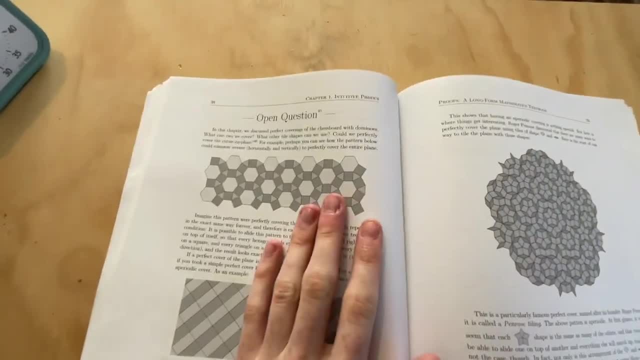 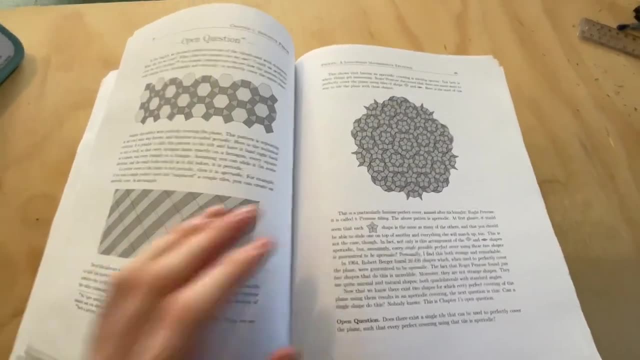 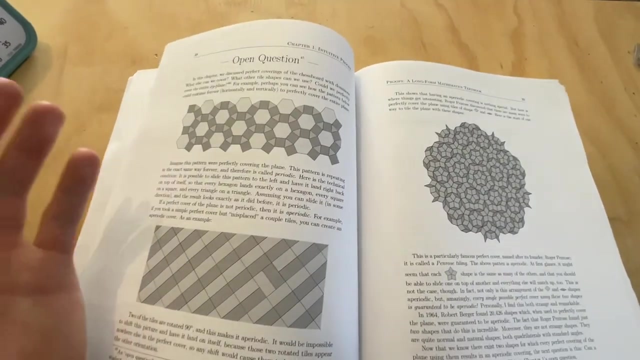 of mathematics. he also has an open question now this is again an incredible additive to, i'd say, any textbook, and he has open questions relevant to the chapter you just did, and these are unsolved questions in mathematics. so it's allowing a the new generation of mathematicians to ponder. 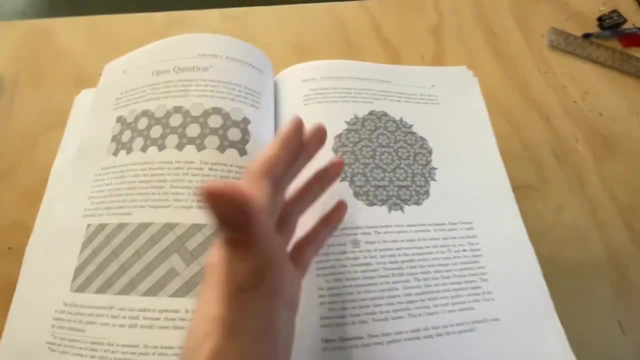 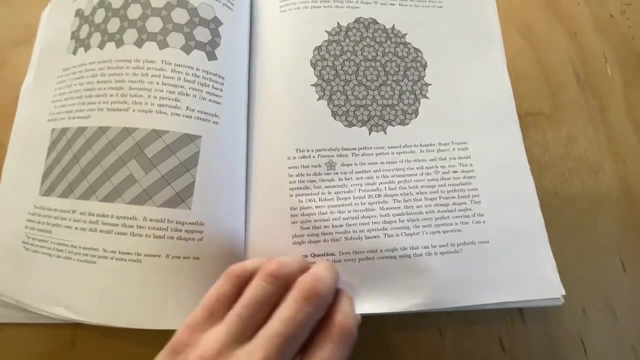 a lot of really cool questions in mathematics and it allows you to do the same. you can read through these and ponder solutions to these unsolved questions in mathematics. here is an example of one of the memes he's added in this book, so it's um describing your journey towards. 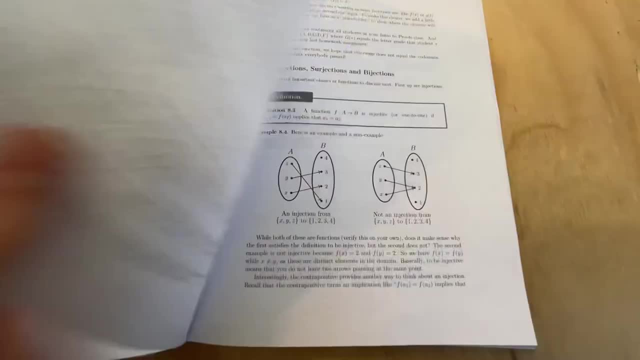 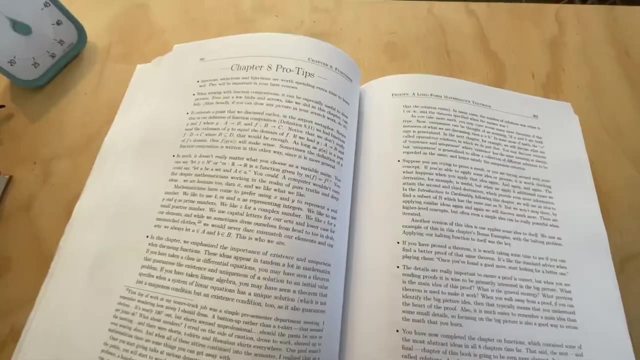 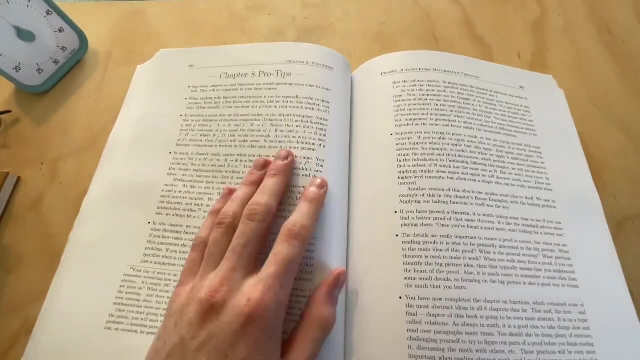 understanding functions. he's got lots of humor in this book, really good diagrams easy to understand, at the end of every chapter. he also has what's called pro tips, so things that he wish he had known when he took this class and learned proofs, and these are actually helpful. a lot of these are actually quite helpful tips. 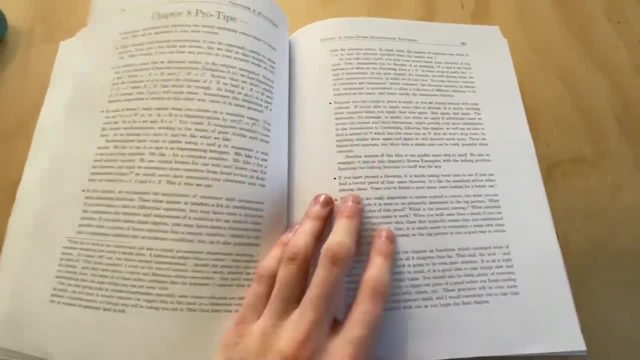 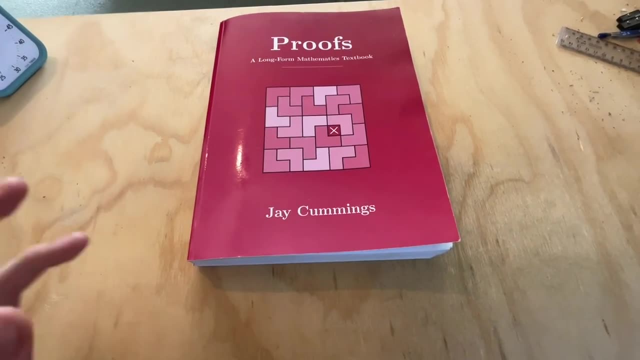 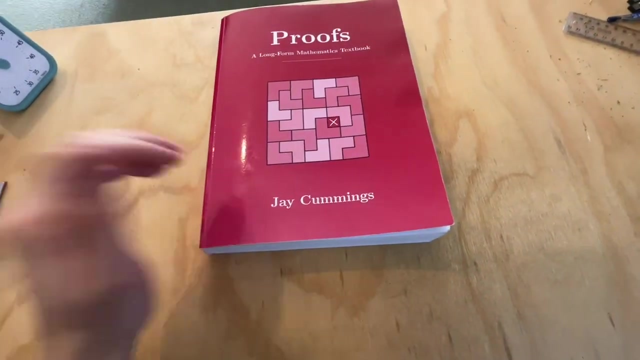 and um, yeah, i think it's another awesome additive to this book. so i highly recommend this book to literally anyone that has any sort of interest in mathematics or mathematical proofs and you have a little bit of a math background yourself. i would 100, 100 recommend you pick this up. it's really cheap. it's really affordable if you can get over the